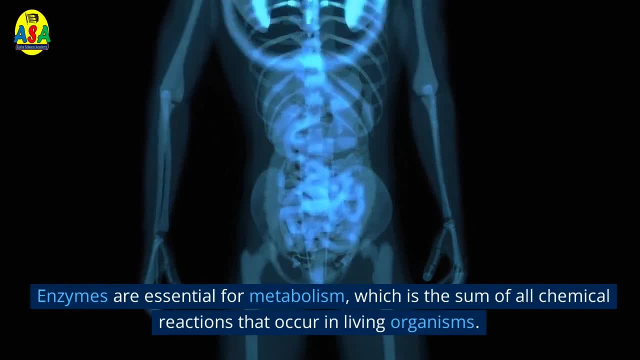 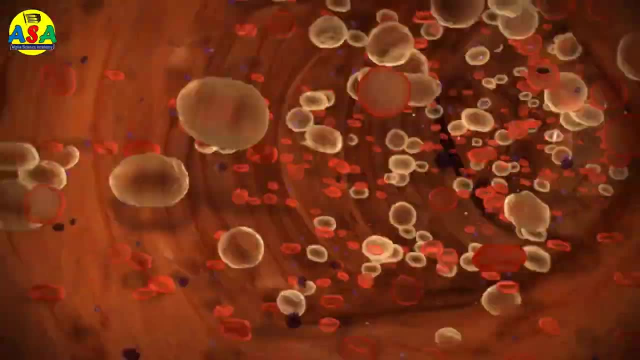 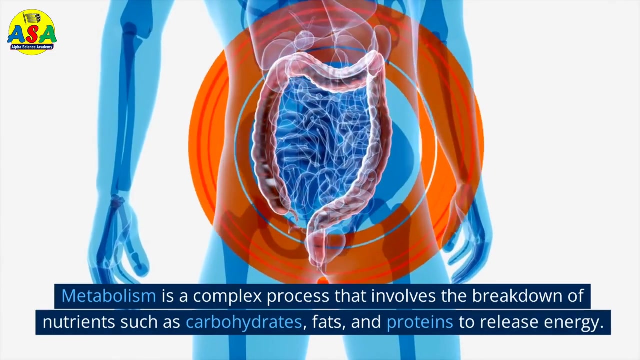 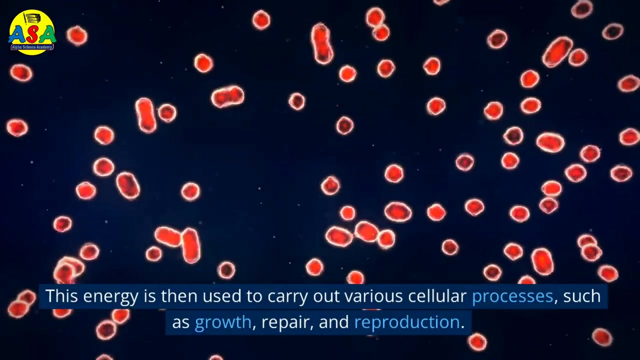 Enzymes are essential for metabolism, which is the sum of all chemical reactions that occur in living organisms. Metabolism is a complex process that involves the breakdown of nutrients such as carbohydrates, fats and proteins to release energy. This energy is then used to carry out various cellular processes, such as growth, repair and reproduction. 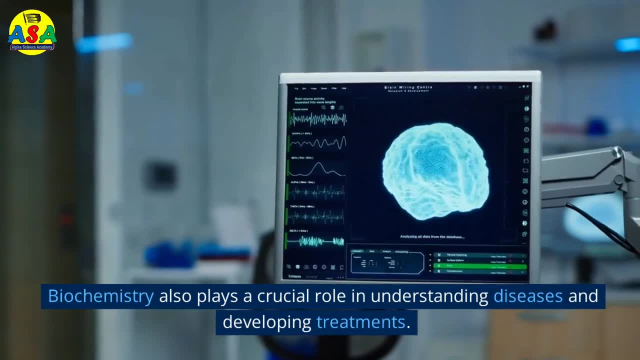 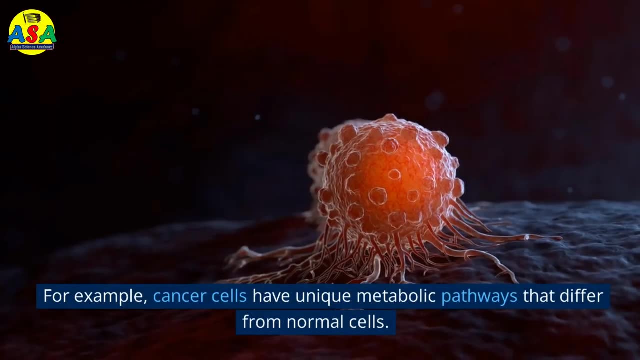 Biochemistry also plays a crucial role in understanding diseases and developing treatments. For example, cancer cells have unique metabolic pathways that can produce side effects. For example, a cancer cell can produce an additional level of chemical responses that can reduce its ability to produce cells. 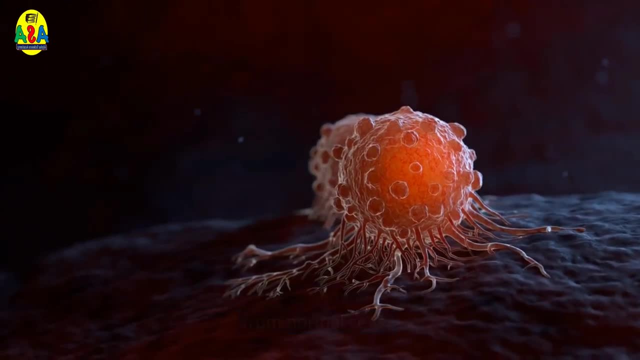 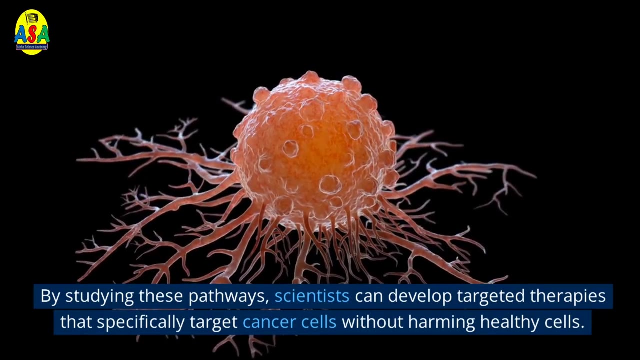 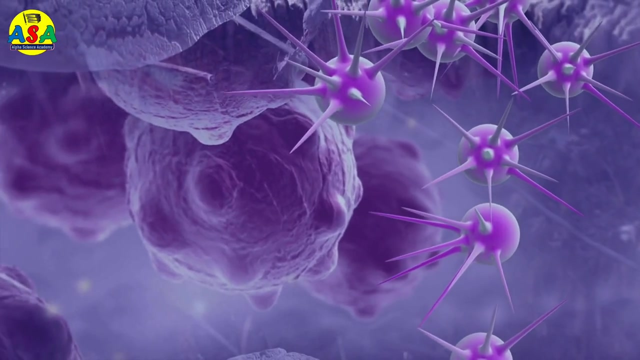 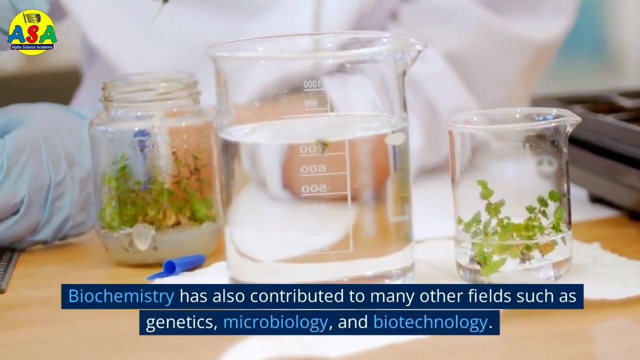 The cell has two types of DNA pathways that differ from normal cells. by studying these pathways, scientists can develop targeted therapies that specifically target cancer cells without harming healthy cells. biochemistry has also contributed to many other fields, such as genetics, microbiology and biotechnology. in genetics biochemistry. 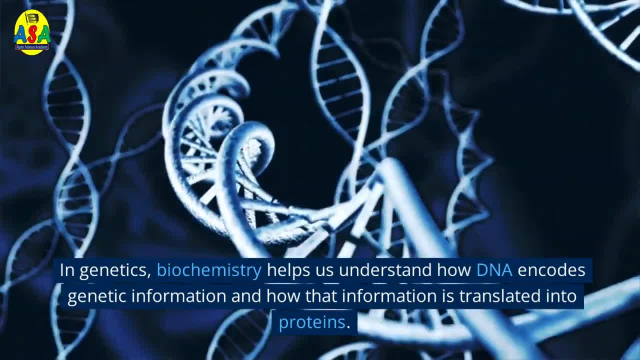 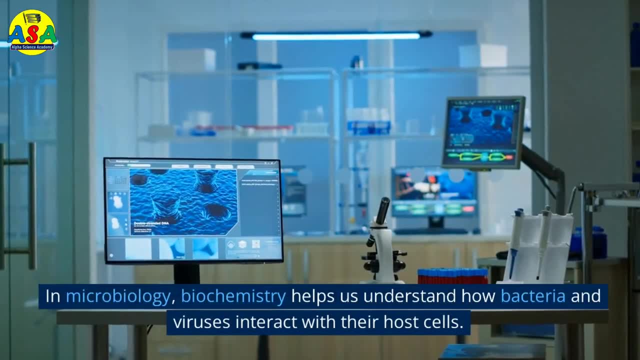 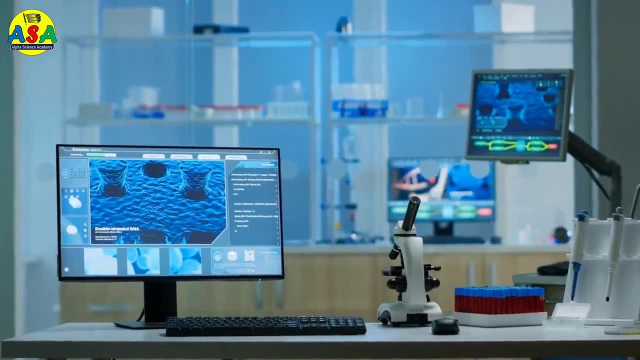 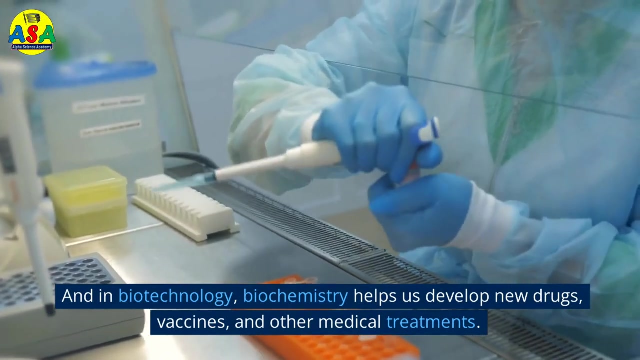 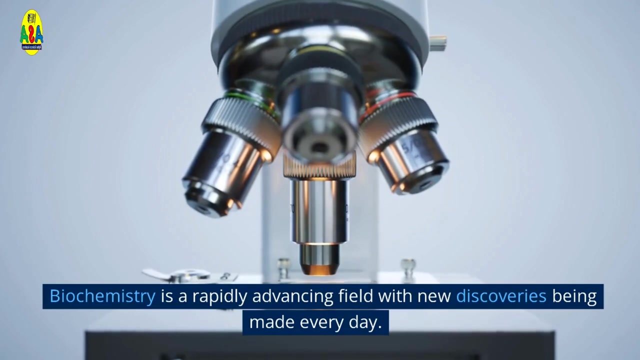 helps us understand how DNA encodes genetic information and how that information is translated into proteins. in microbiology, biochemistry helps us understand how bacteria and viruses interact with their host cells. and in biotechnology, biochemistry helps us develop new drugs, vaccines and other medical treatments. biochemistry is a rapidly 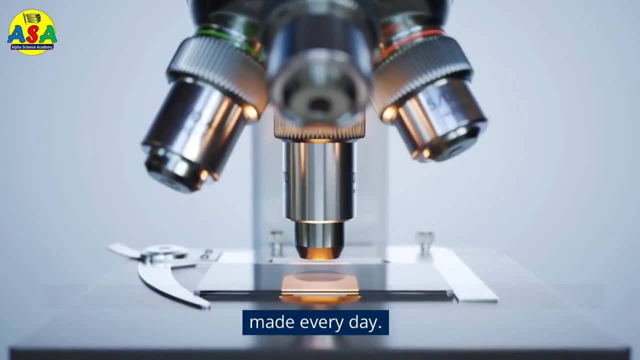 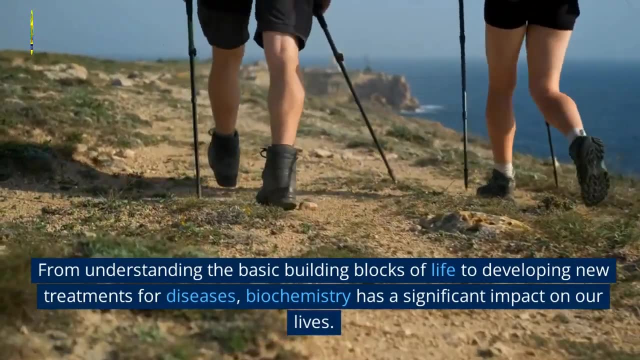 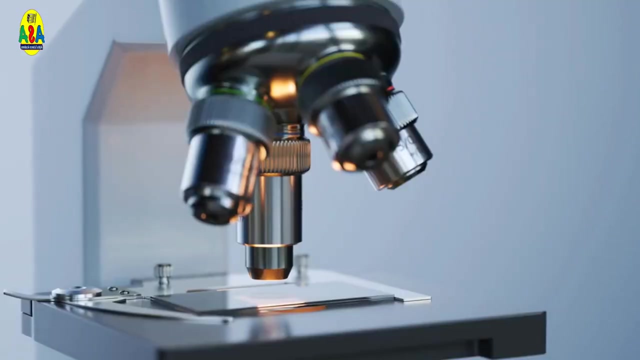 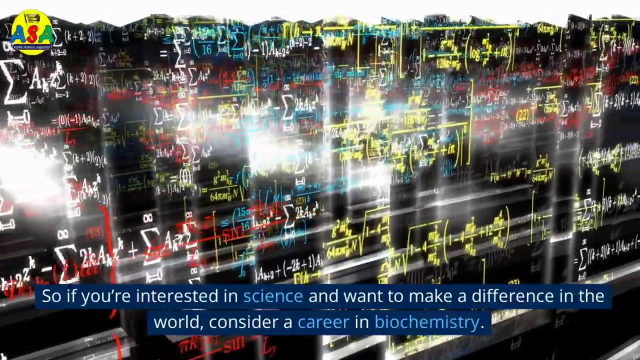 advancing field, with new discoveries being made every day. from understanding the basic building blocks of life to developing new treatments for diseases, biochemistry has a significant impact on our lives. so if you're interested in science and want to make a difference in the world, consider a career in biochemistry. 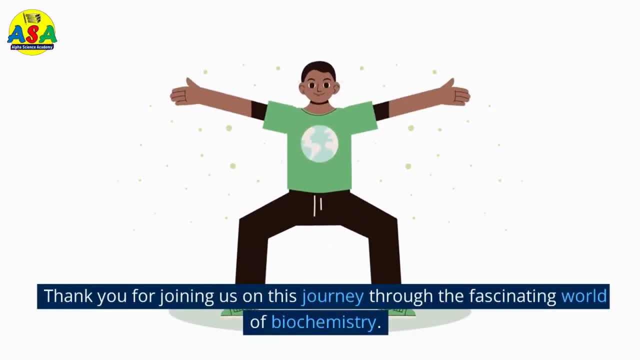 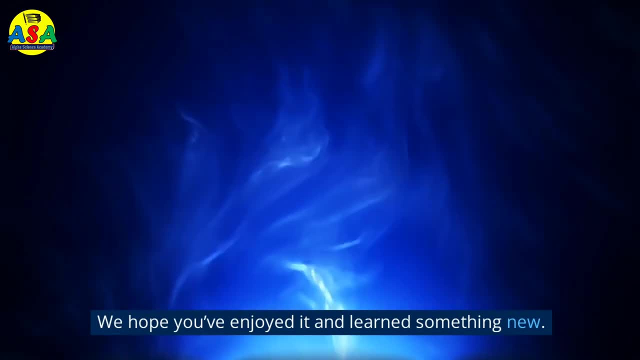 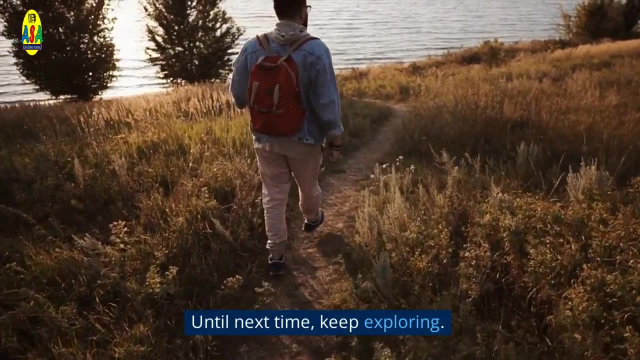 thank you for joining us on this journey through the fascinating world of biochemistry. we hope you've enjoyed it and learn something new. until next time, keep exploring you.